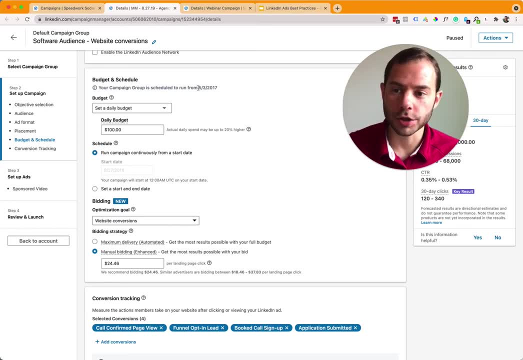 Hey guys, Anthony here from SpeedWorks Social and one of the most common questions I get from people is asking about what is a typical budget and how do I set up my bidding for LinkedIn ads. A lot of people get to this section here- budgeting and schedule and bidding- and they're wondering what to put in here On LinkedIn. there's a lot of different settings here that you can select between: conversion, landing page clicks, what do I set my daily budget to? what do I set my bid to do? I use automated bidding. There's a lot of questions people have when they get to this section, so I'm going to walk you through some best practices. 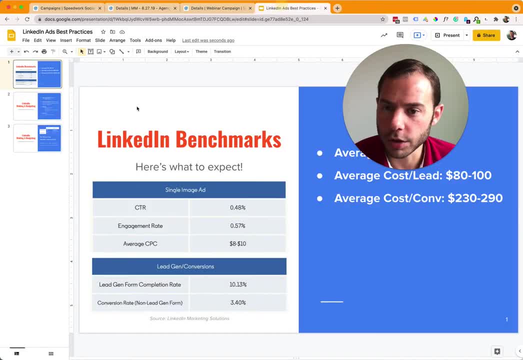 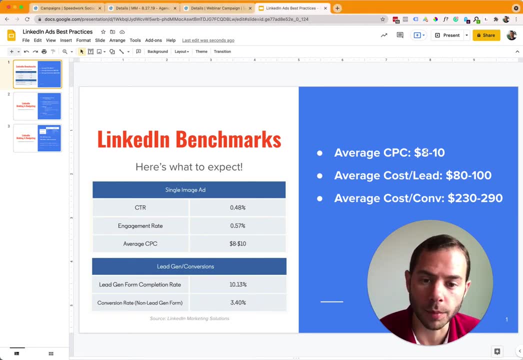 here and how to get the most out of your campaign. So first thing is some benchmarks that LinkedIn publishes. So if you're using LinkedIn, LinkedIn has premium traffic. they know they have high level professionals that can be very valuable to target, So you're going to pay for those targeting options. The average CPC on LinkedIn in the US targeting middle management, is about eight to 10 bucks. If you're outside of the US, that's tends to be significantly lower. And then if you're targeting entry level people, this might be lower. And if you're targeting very high level people such as C suite and owner. 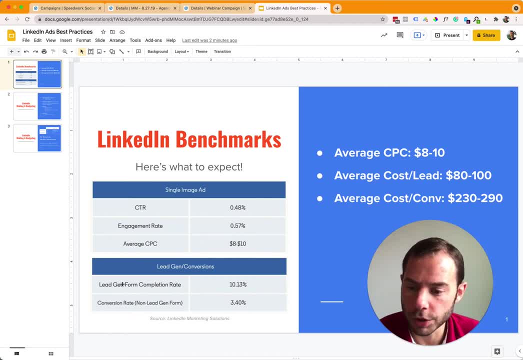 this is going to be even higher. These are some metrics that LinkedIn publishes. The average complete conversion rate over here for lead forms is about 10%. The average conversion rate for not lead forms is about 3%. So just showing that this gives you some average metrics- that your average cost per lead can be in the 80 to $100 range, And then your average cost per conversion on a website- if someone's going to a website to fill in a form, that might be in a 230 to 290 range. So that's pretty high. So there's some things that we can do to make sure we're getting the best performance out of these campaigns And to 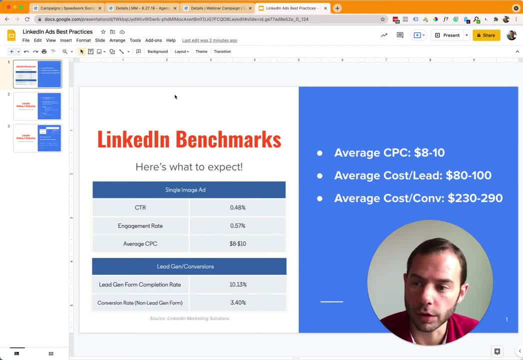 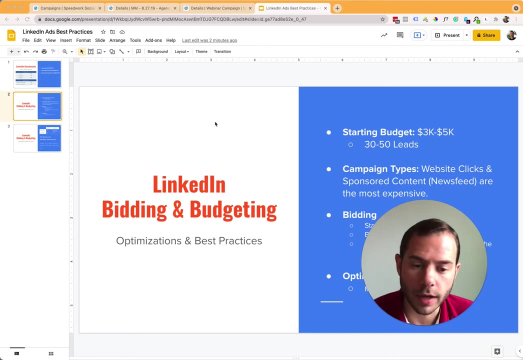 some different optimization optimizations you can make. So I'm going to walk through here some of those tips, But this is kind of just to set the stage of where you're probably going to land in terms of costs and why you want to make some decisions. So the first thing here is the first thing to think about is kind of what's your starting budget going to be? And with those high CPCs you're going to need a higher starting budget than, say, a platform like Facebook or Google just to test some stuff out. So we usually see that most people want to start with at least 3000 to 5000.. And ad spend: 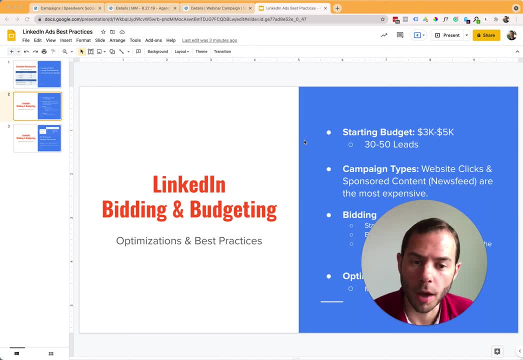 over a time range, and that can be over one month or it can be over a couple months. But you know, when you set up your campaigns you'll want to split test your audience targeting, you'll want to split test an offer and then you want to split test ads. This is generally the 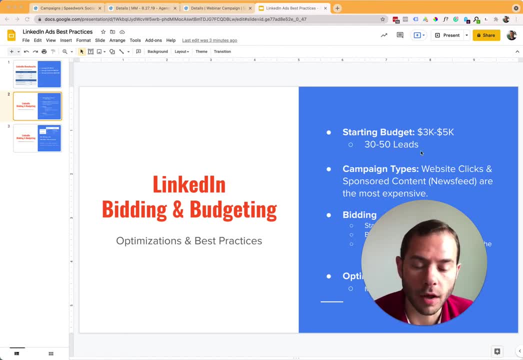 amount of budget you'll need to cover those split tests and then to drive. to drive a significant number of leads that you can start evaluating. you know what's the quality of leads and make some optimizations based off that. you know most companies are going to need to drive. 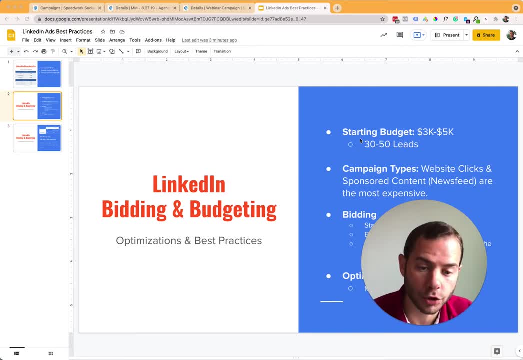 a large number of leads. you know, depending on what your conversion rates in your funnel look like, companies will need to drive a higher number of leads to then convert a certain number of those into customers for their business. So some things that we typically see is campaign types First, 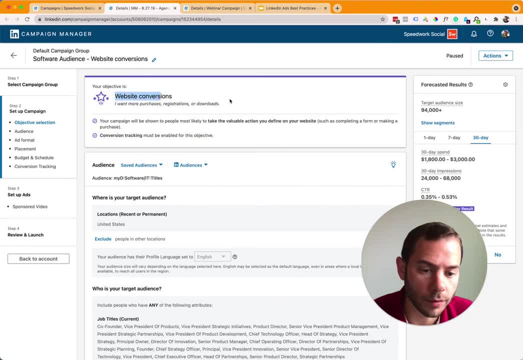 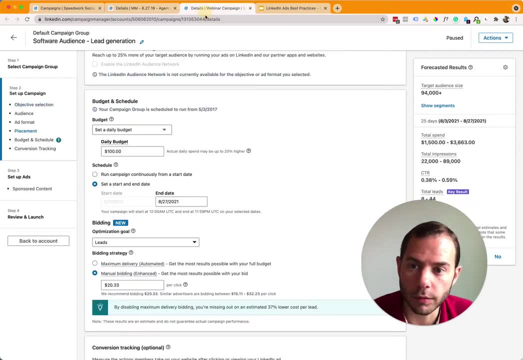 thing that you're going to select when you're setting up your campaign. you're going to select what type of campaign you're creating, And it's important to note that website conversions or website visits, are more expensive than the lead generation objective or other types of campaign. 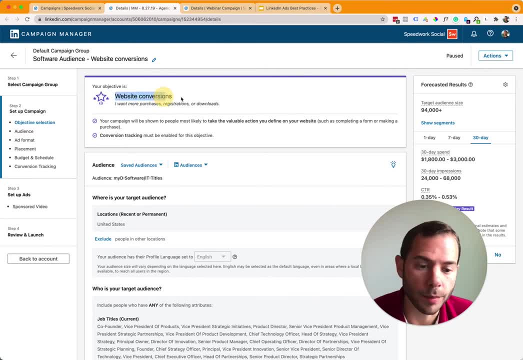 objectives And the reason is because on LinkedIn, if you're taking people off the platform, they're, you know that's kind of less valuable to them because that they have less of an opportunity to serve people as in the future, Whereas if you use a objective like lead generation, people are. 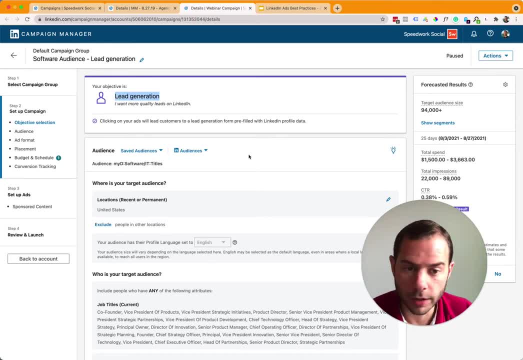 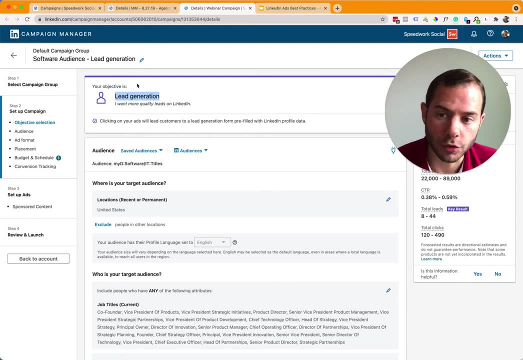 staying on the platform. they're opening up the form there And LinkedIn has, you know, more opportunities to engage them and have that user be active afterwards versus leaving the platform, So that user is more valuable to them. So they give you a little bit of a discount in those. 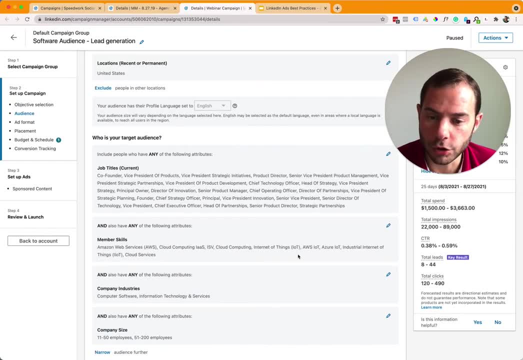 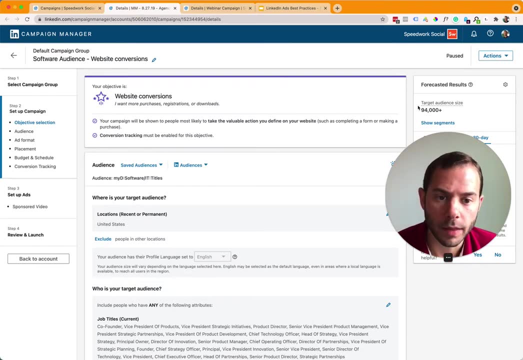 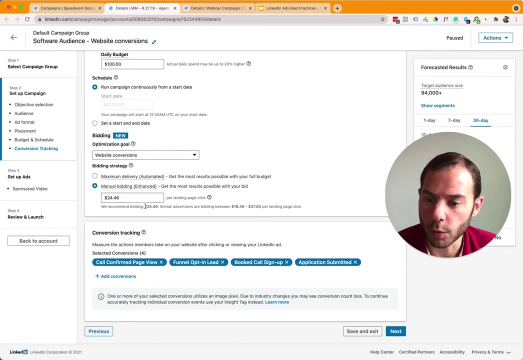 costs. It's interesting to see. you can see here I have two identical audiences of the same size here that I was, you know, mocking up to show this- that same size. come down here to the bidding section For website conversions campaign. here you can see that the we were the average bid is. 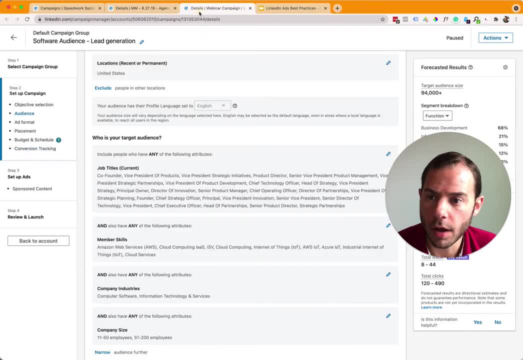 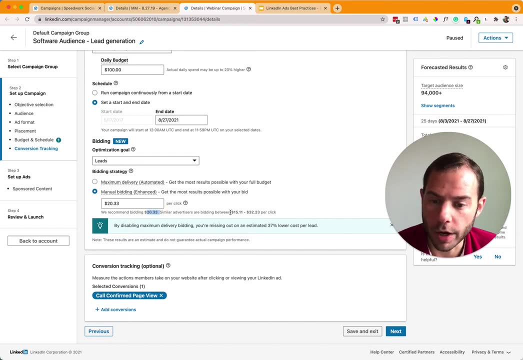 2446. And then the range is from 18 to 37. But over here when I go to lead generation using the same audience, if I scroll down here, the average bid is 20. And the range is 15 to 32.. So in that, 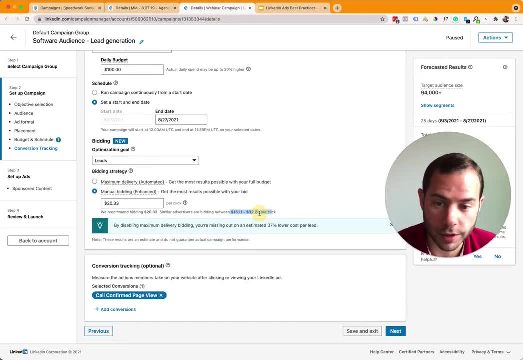 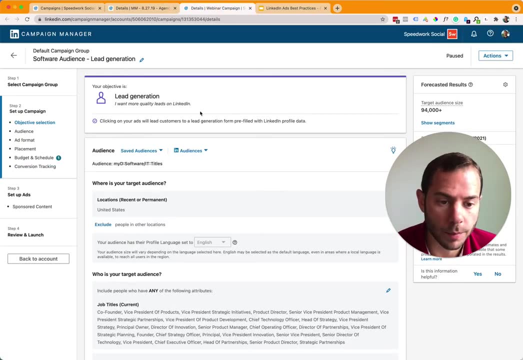 difference there? that's about a 20 to 25% difference, which is pretty significant when you look at your ad unit. So you know, if you're comparing campaign types, consider using lead forms, because they're going to keep people on the platform. And then the other thing is when. 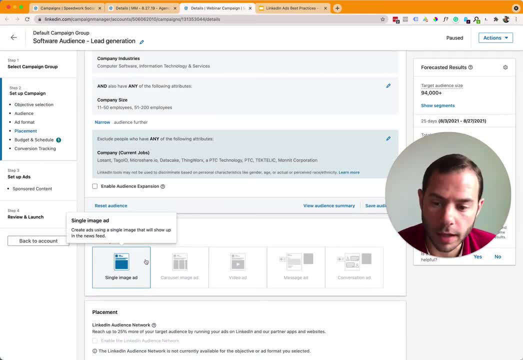 you're selecting your ad unit. sponsored content here in the newsfeed tends to be the most expensive because that's the highest quality ad unit. everyone's bidding on that space, So that tends to be the most you know, the most competitive and the most expensive. Consider you can consider. 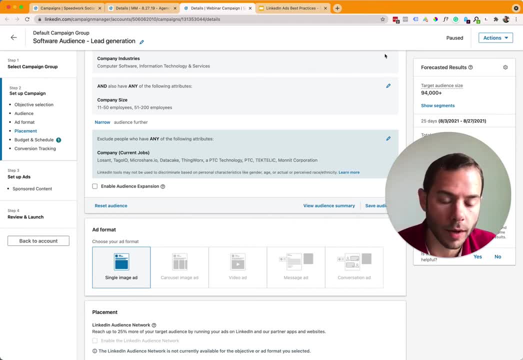 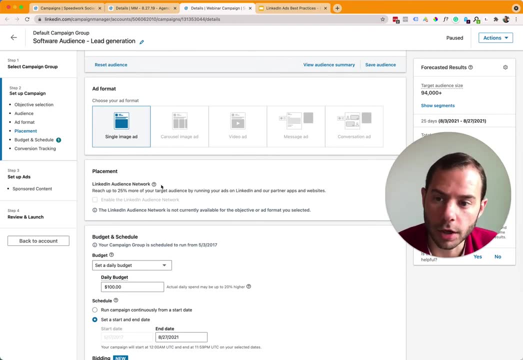 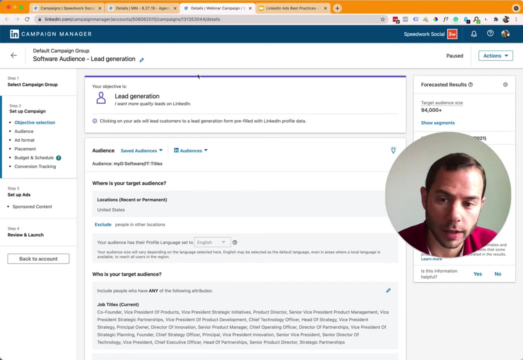 text ads and dynamic ads as smaller ads that show up in the sidebar, the newsfeed. those tend to be the whole. So if you want to, just you know, start out by testing something you can either test using the lead generation objective or you can test using text ads and dynamic ads for a cheaper way. 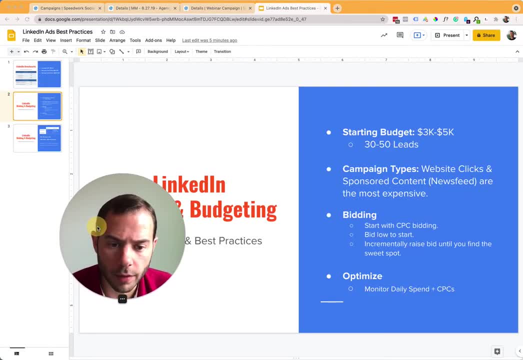 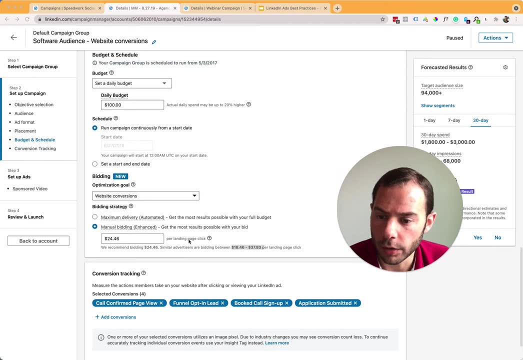 to get started on LinkedIn. So some other things to think about is when you're starting your bidding. So first is the bidding type that you want to select over here. the options they give you is maximum delivery, automated or manual bidding, enhanced. And the thing to know about this here: 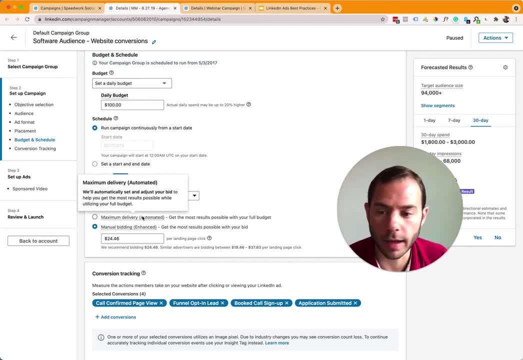 is that automated bidding is actually a CPM bid and you're kind of letting LinkedIn set your bids for you based on some of these averages here, And then manual bidding is where you're going to set the bids yourself and say: I'm not. 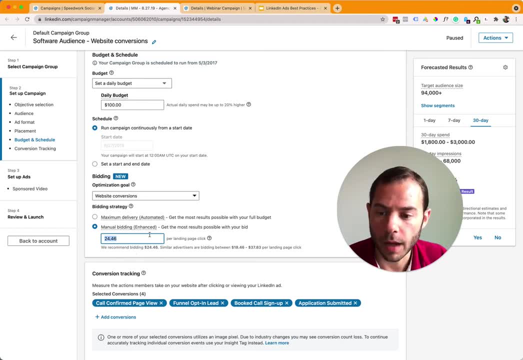 going to pay over a certain amount for clicks, And this is a per click bid. So this is a CPC bid And the top one here is a CPM bid. So it's important to know those differences. So there's a few. 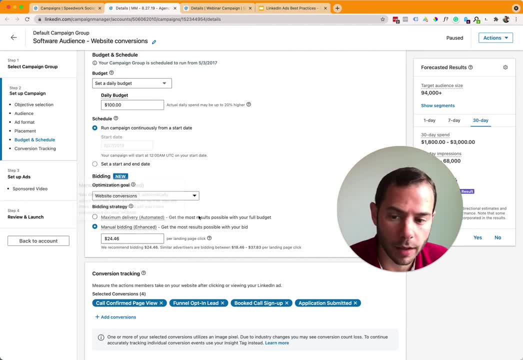 you know most people, we recommend starting with a CPM bid. there is a case when an automated bid does work, And I'll talk about that in a second- But manual bidding- you want to pay for every click to start And you know LinkedIn is showing. 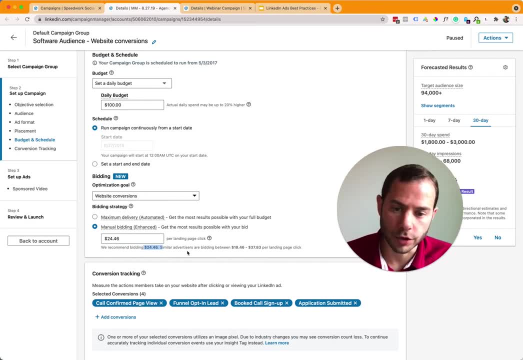 you these ranges here, And these ranges include all the advertisers on the LinkedIn platform, including some very big companies. And very big companies have very big budgets And you know the higher value that these prospects are to them, the more that they're going to pay to bid on them. 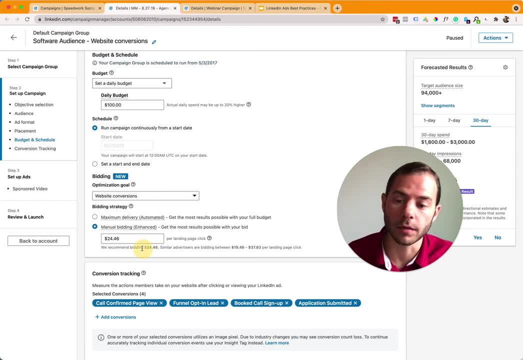 So big companies, big budgets, are spending a lot of money on LinkedIn, And that's where a lot of these high costs come in too. So you know, if you are a small, smaller advertiser and you're not, and you don't have a million dollar budget. 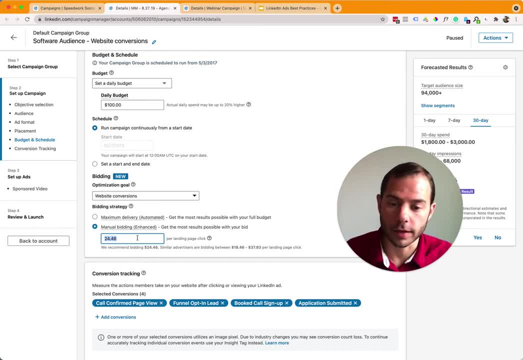 you know you probably want to start and you want to optimize your costs at this section. So it's important to note LinkedIn is going to: if you select manual bidding, LinkedIn is going to start by popping in what's the average bid here to give you that. But you 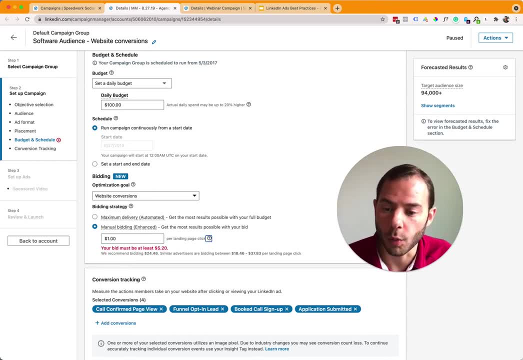 can set this value. So usually I'll come in here and I'll start by finding what's the low, what's the real low of this range. If you put in a low number here, LinkedIn is going to tell you where the actual floor is for this audience. We see in the US the actual floor tends to be: 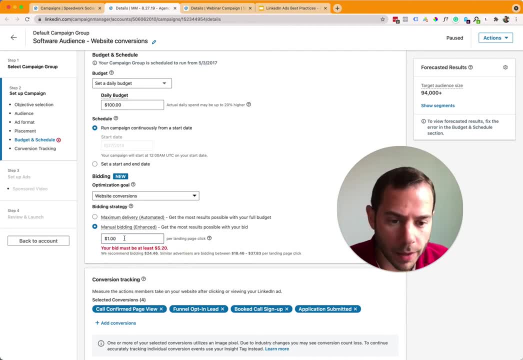 three to six bucks. And keep in mind you know this is a bid, So you are entered into an auction. If your bid is too low, you're you just won't get any impressions. LinkedIn won't serve up your ad. 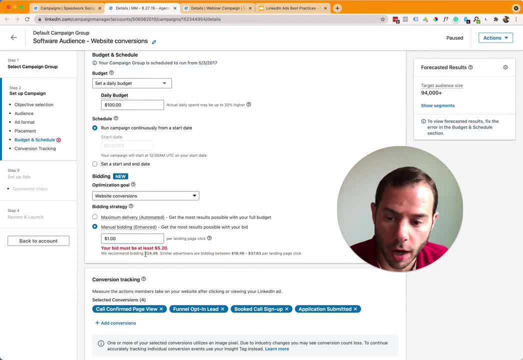 So this, this bid does need to be high enough for you to get some, some traffic there. So it's interesting to see. you know, I put in one. it tells me the actual floor is five bucks here for website conversions. You know they say the range is 18, but the floor is really 520.. And if I come, 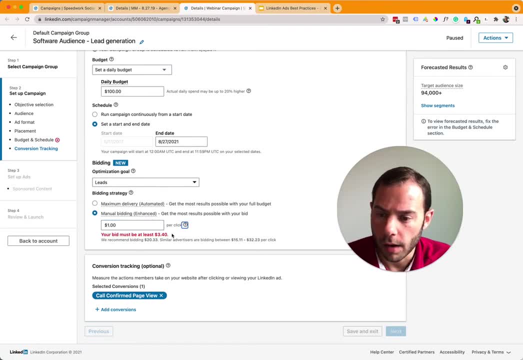 over here to the lead generation one, and I do the same thing. if I put in one, let's say, the actual floor is 340.. So there again you can see that there's a significant difference between lead generation clicks versus website clicks. But where I'll usually start is 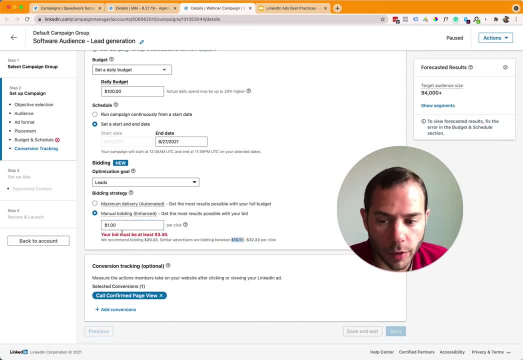 I'll look at what the what the range is And I'll usually take the low end of the range And I'll usually look at the floor here and also evaluate my audience. If I know I have an entry, more of an entry level audience, I might start at like 10 to 20% over this floor. So if I have an entry, 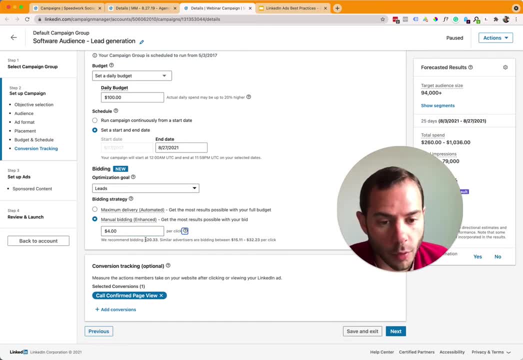 level audience. you know I might start with just a $4 bid here, because I know that these are going to be some. if it's an entry level audience, those should be some cheaper clicks. But if I know I'm targeting middle managers or VPs or owners, then I'm probably going to start at about. 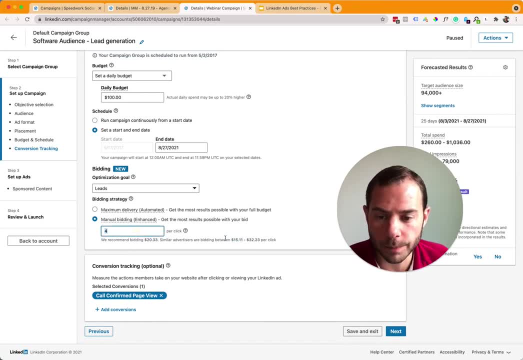 half of what this range is, of what this low end of this range is. So at 15, you know I might start at seven or $8 per click. Usually I'll start probably at seven. I'll, and I'll monitor the campaign as it runs to make optimizations. So know that you have a range here and this is all. 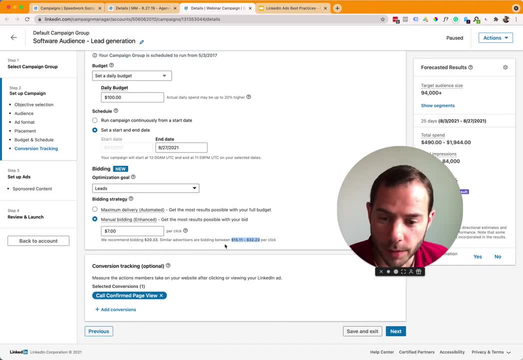 advertisers on the LinkedIn platform, including some very big companies with very big budgets. That's why this range is so high. If you're a smaller advertiser and you're spending, you know, in the thousands per month, then you're probably going to want to set manual bid and set a very low bid here to start. 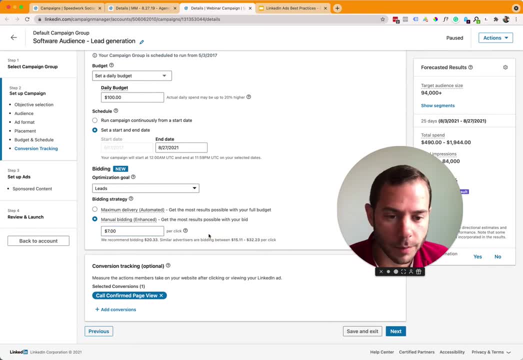 We also see that you know, bidding low doesn't necessarily mean you're going to get worse traffic. We see, we see a lead quality tends to hold pretty well that you're going to get just as good of people when you bid low. But you know, no, as your campaign runs. 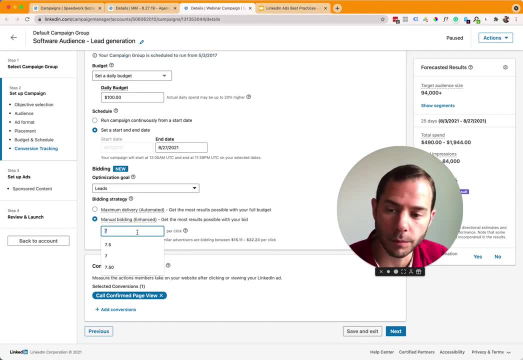 you might exhaust the cheapest people at some point And then you'll need to eventually raise your bids. So this is something that you can do over time. You know other things you can do is refreshing, creative, maybe expanding your audience. but you know, starting with lower bids is going to make. 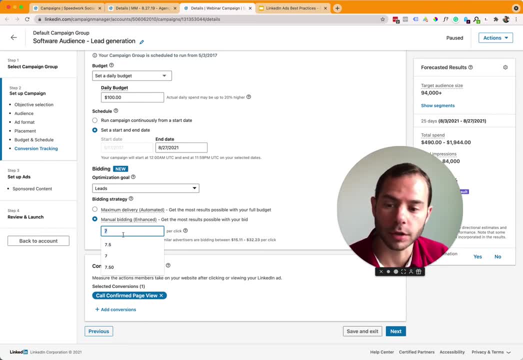 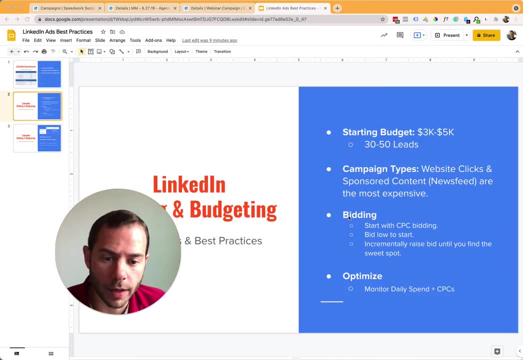 LinkedIn target the lowest hanging fruit And then you might need to consider raising them slowly after that. So this is something you might need to come back to at different times. So back to my notes here: bidding: you want to start with CPC bidding. bid low to start. 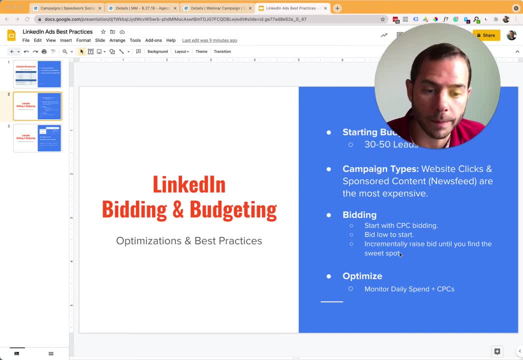 and then increment incrementally raised bids until you find your sweet spot. And the thing about this is on a day by day basis or over a certain time period you can look at. are you spending your full budget every day? If you're not, then you might be bidding too low. 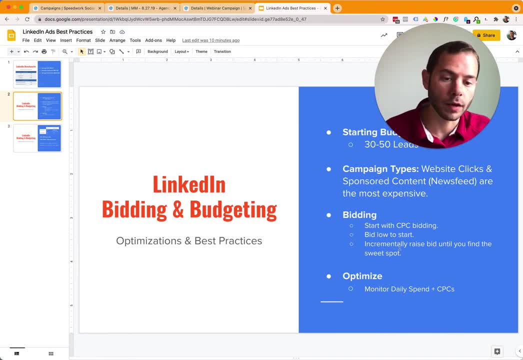 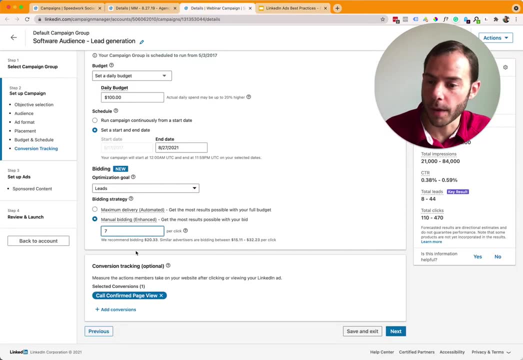 And you know, the sweet spot that we talked about here is when you're spending your full budget every day, Um, but not over that. So you know, if I, if I, if my budget is only a hundred bucks per day and I and I do bid 20 bucks, then you know, in five clicks I'm going to exhaust my 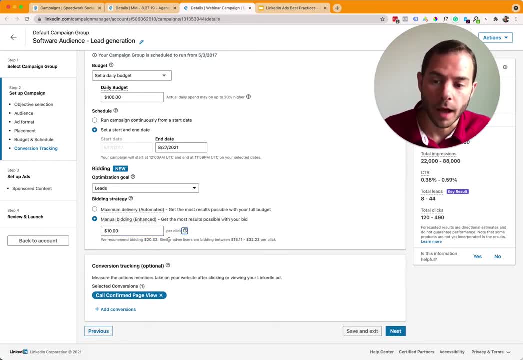 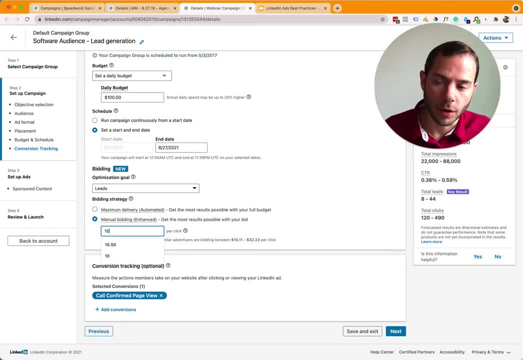 then maybe I do need to increase this by just a little bit. Um so, keep an eye on: are you spending your full budget every day? If you're not, then you might need to raise your bid to to reach that, because because the low bid might be holding you back from getting impressions. 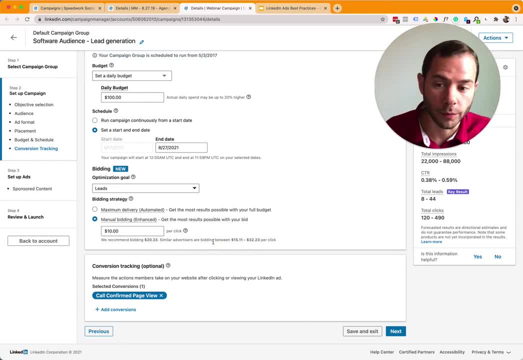 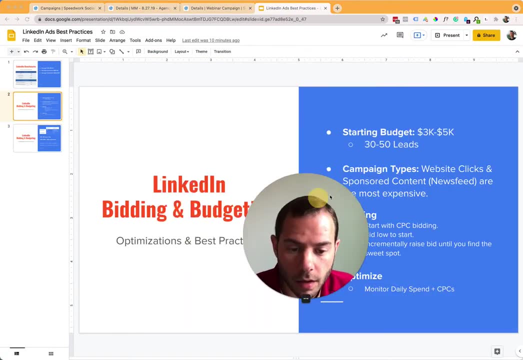 and you know serving Um, and then if you are spending your full budget early in the day, then you know you're probably overspending for those clicks, So you can then lower your bid from there. Um. so that's how you do optimizations there, And usually I'll come in, you know, and as a campaign. 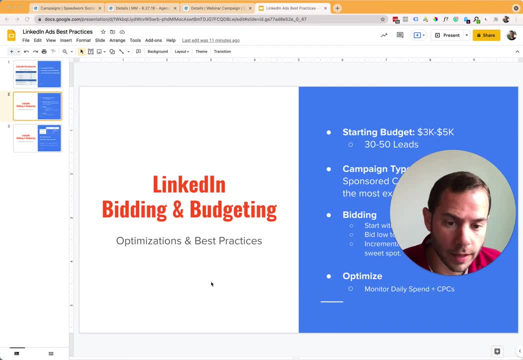 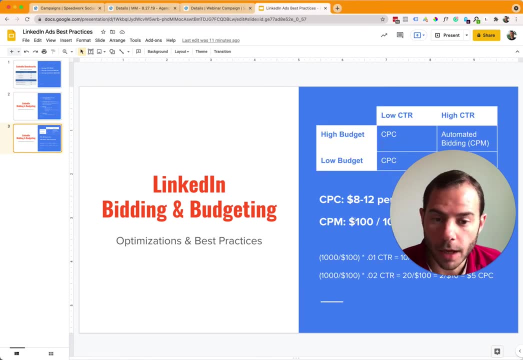 launches. I'll come in, maybe on a daily basis or throughout the periods of the day, um, to see: is it on track to spend the full budget? Am I overspending? Is there optimization, optimizations that I can make? So next one, here is getting a little more advanced, Um. so there is times when 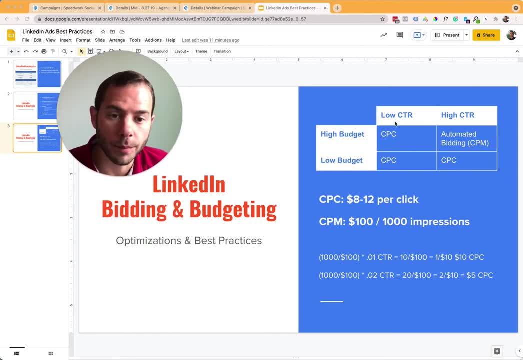 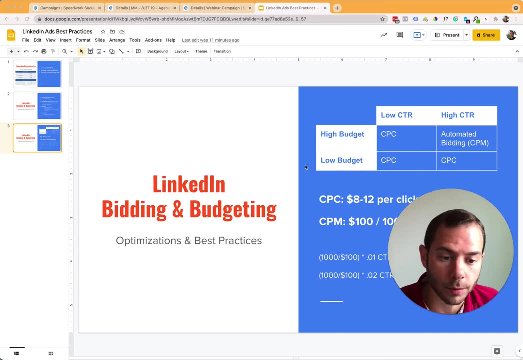 automated bidding is useful and you can see this little chart here that compares your click through rate to your budget. So in most cases you do want to start with a CPC bid because that's going to give you the most optimal Costs on LinkedIn, Um, where if you have a low click through rate, you want to be on CPC If you. 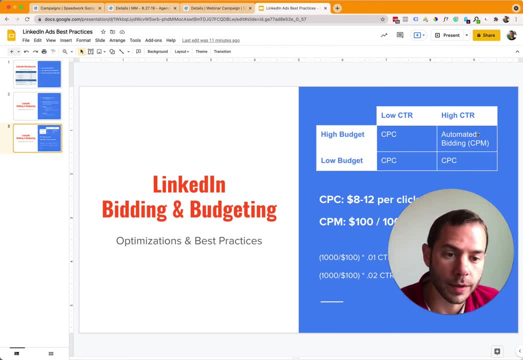 have a low budget. you want to be on CPC. The thing is, when you go to a CPM bid, you're paying per impression. So if you have a very high CTR on your ads, whether you know your ads are just working. 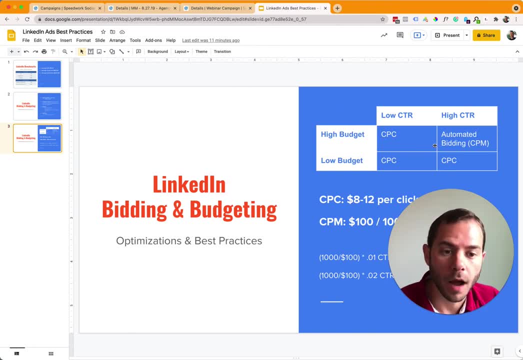 really well or people are very interested in what you have to offer. Um, if you bid by impression and if you have high CTR rate, you're going to get more clicks for cheaper. Now, the reason why low budget and a high CTR are still CPC is because LinkedIn does have. 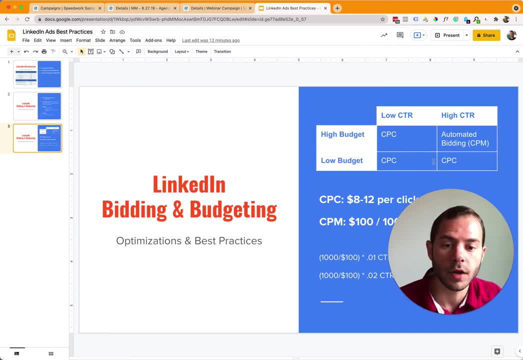 A wide range of people on the platform, that can be very expensive. So if you have a low budget and you set automated, you know LinkedIn might go from one CEO and one manager of a person and you might still spend 50 bucks in that clip for that CEO. When, if you have a very low budget, 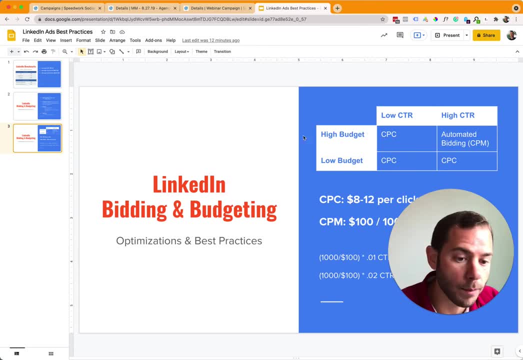 you want to be as efficient as possible. So if you have a high budget and you're trying to maximize your traffic- you know you're trying to maximize your clicks and you're trying to, you know, reach as many people in your audience as possible- You do have a high CTR- then you're going to be 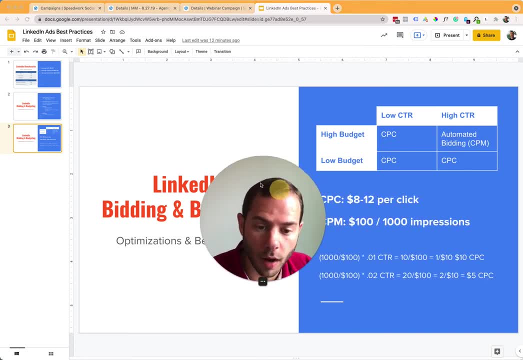 and that's going to be advantageous to use automated bidding for you, And I'll show you why. if you look at some of the math here, CPCs on LinkedIn tend to be between eight to 12 bucks per click and you know average CPC range is about a hundred bucks for a thousand. 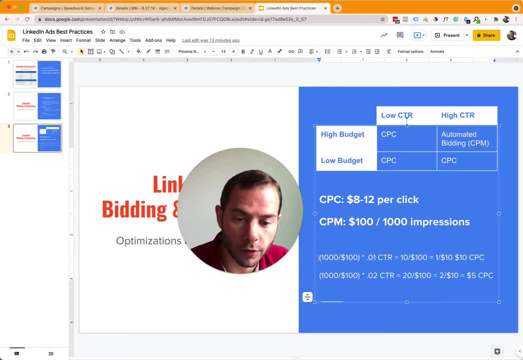 impressions. So you know this line here, this first line here is: if you have a thousand impressions and a hundred bucks and a you know say, a 1% CTR, then you're paying. you know, maybe a dollar, you know you're paying about 10 bucks per click here, But then if you have a $2,. 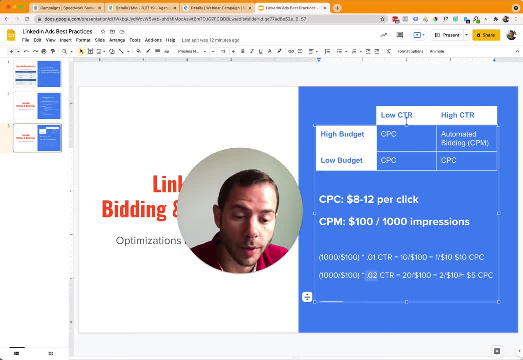 if it, if you have a 2% CTR, then suddenly you're paying about five, five bucks per click Here. So we usually see around 0.8 is maybe when it starts to make more sense to do automated bidding, And again for only for high budgets, And if you're over, if you're over one, that's again. 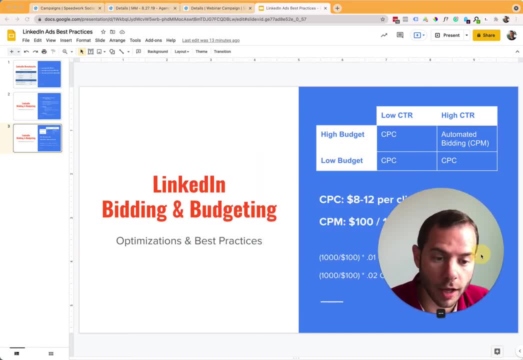 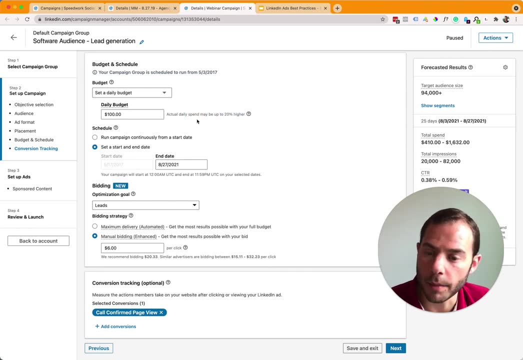 a time when you want to look at switching to automated bidding to get the most out of your campaigns. A couple other random notes is when you set your daily budget, LinkedIn can spend up to 20% higher And it kind of makes sense if they're serving a whole bunch of impressions. 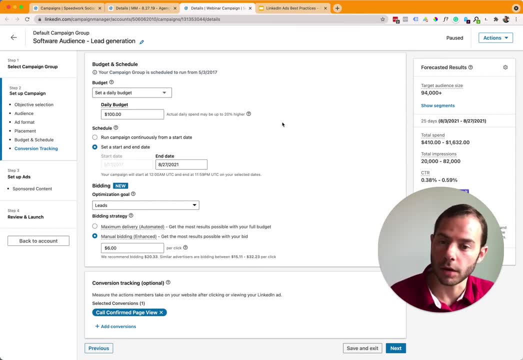 maybe a couple of people click at the same time And then you know then you're going to get charged a little bit more. but keep an eye on your budget And if it's a problem then maybe bid have have your budget be about 20% lower. but we don't usually see it's an issue. You'll. 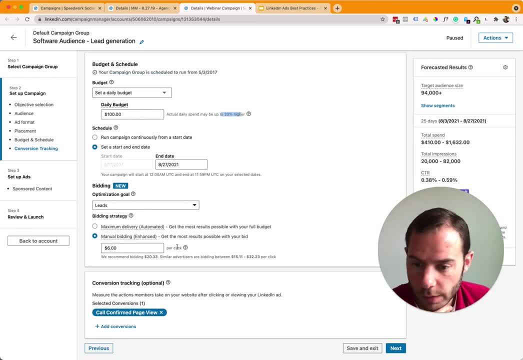 just know that some days you might be 20% over that budget And also coming down here on a per click basis, this enhanced part here, uh, you can see that they say they can bid actually 45% higher, um than what you set here. So, on a daily basis, another thing that you can do. 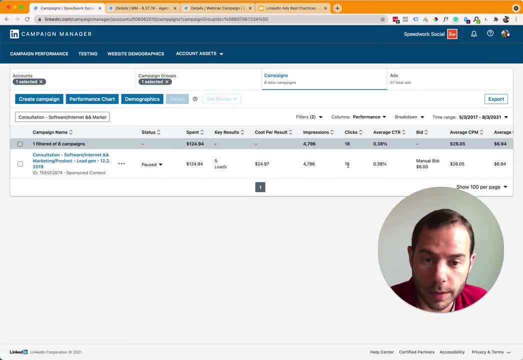 is: keep an eye on what is my actual CPCs that I'm paying. So if I'm bidding here, I'm going to be charging a little bit more. but keep an eye on what is my actual CPCs that I'm paying. So if I'm bidding here, I'm going to be charging a little bit more. 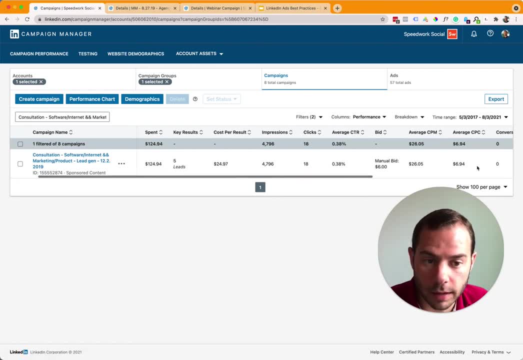 and I can see that my actual CPC is actually 694.. This is LinkedIn. um, you know, using that enhanced bidding to bid slightly over what I am bidding And then, if I can see that, you know, if I see, if my bid six and we're consistently getting, you know, almost seven bucks per click. 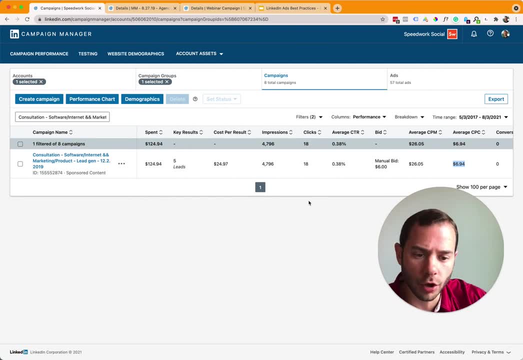 that means LinkedIn is kind of stretching or having to stretch to go to, to get impressions and to get clicks. So something to keep an eye on is if you're not spending your full budget every day and you see your average CPCs are above your average CPCs, then you're going to be 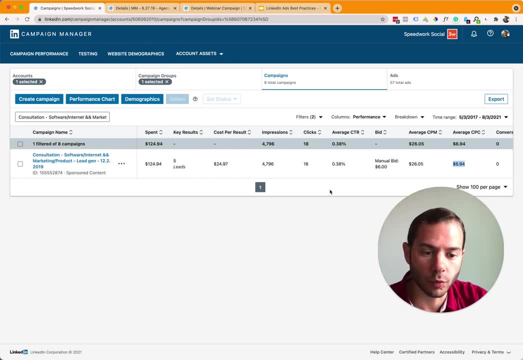 spending your full budget every day. So that's an indicator of when you need to increase your CPCs, increase your bid, Uh. and then again, if you see that your average CPCs are actually significantly lower than when you're bidding, um, and you are reaching your budget every day. 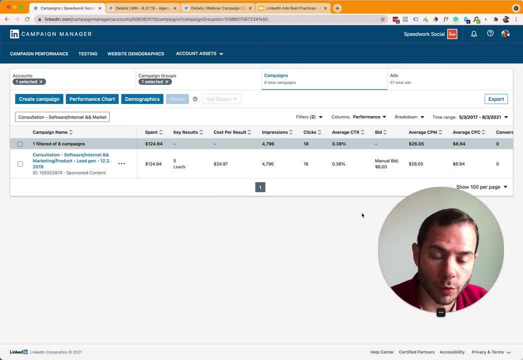 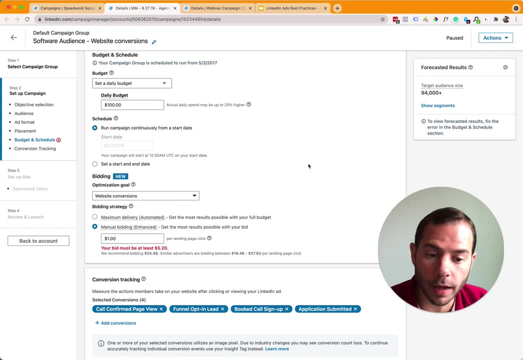 then that's an opportunity to decrease your bid and be more efficient with your clicks and just go after those cheaper, those cheaper clicks there. So that's kind of a lot of info about setting up your bidding and budgeting on LinkedIn ads. My name is Anthony from.